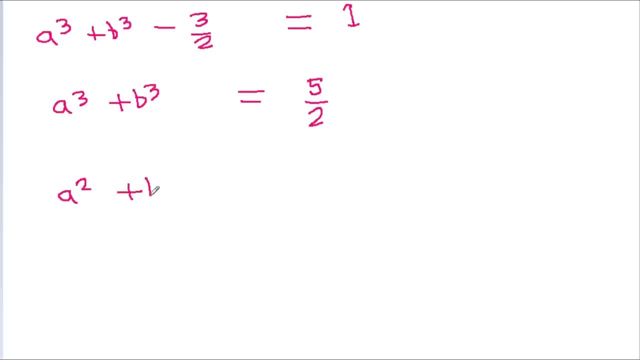 and we have given that a square plus b square is equal to 2, so if we multiply a cube plus b cube and a square plus b square, then a cube plus b cube is 5 by 2, and a square plus b square is 2, and a cube times a square is a power 5,. 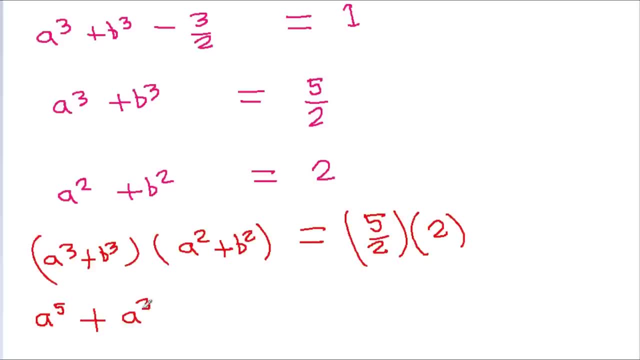 minus a cube times b square is a. cube b square minus b cube times a square is b. cube a square minus b cube times b square is b power 5, that is equal to 5 by 2 times 2 will be 5,. 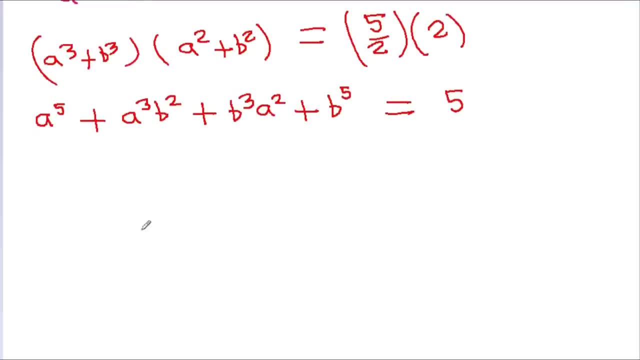 and it is a power 5 plus b power 5 plus a cube: b square plus b cube, a square is equal to 5, and a power 5 plus b power 5 plus, and here we can take a square, b square, common. 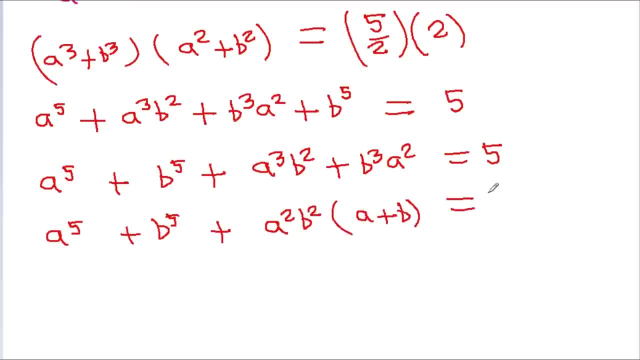 and we will get a plus b. that is equal to 5, and it is a power 5 plus b, power 5 plus a square b square is a b whole square times. a plus b is equal to 5, and a power 5 plus b. power 5 plus a, b is equal to minus 1 by 2 s square. 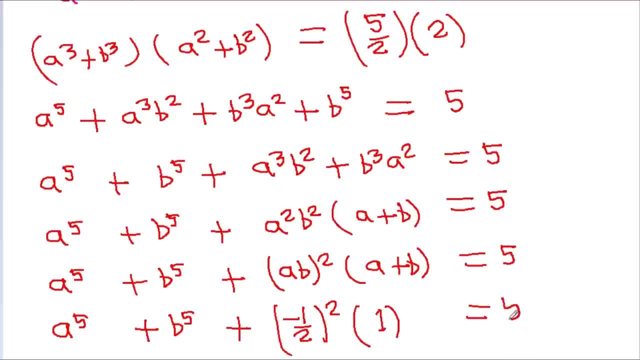 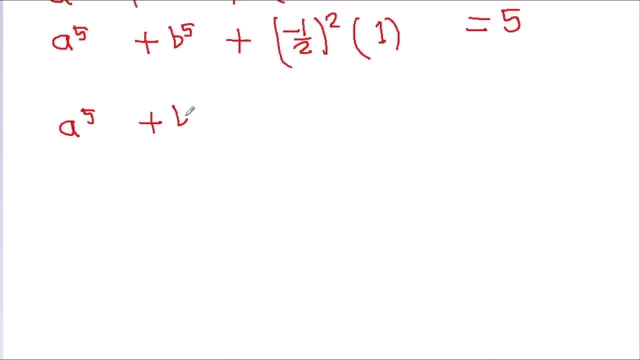 and a plus b is equal to 1,, that is equal to 5, and it is a power 5 plus b power 5 plus minus 1 by 2 s square is 1 by 4,, that is equal to 5,. 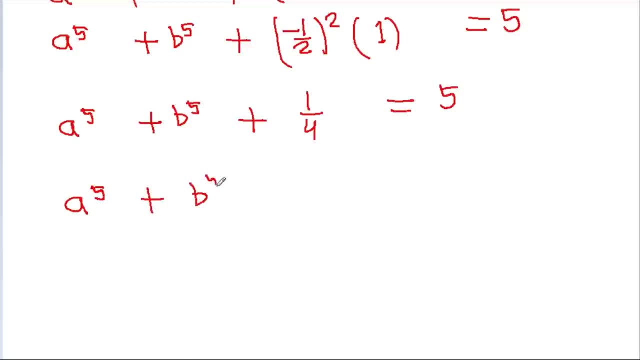 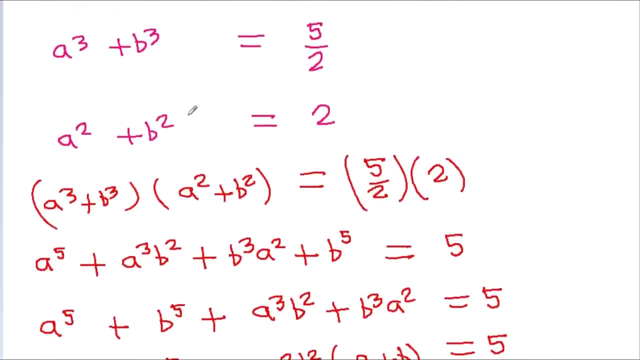 and we get a power 5 plus b power 5 is equal to 5 minus 1 by 4 will be 19 by 4.. Suppose this is equation 1.. and we have a cube plus b cube is equal to 5 by 2,. 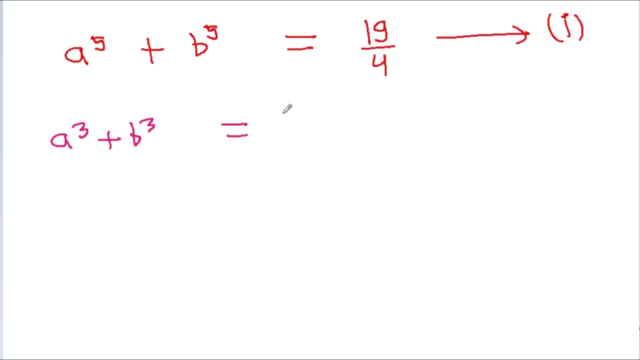 we have a cube plus b cube is equal to 5 by 2 and if it is squared it exist at both side. then we get a cube plus b cube: whole square is equal to 5 by 2 square and a cube square is a power. 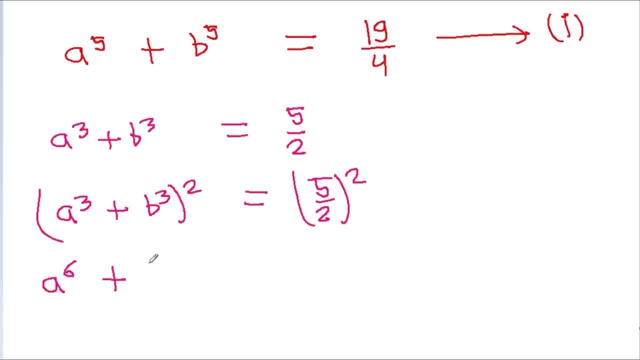 a power 6 plus b cube square is b power 6 plus 2 into a cube. into b cube is equal to 5 by 2 square multiplied by 25 by 4, and it is a power 6 plus b power 6 plus two times. 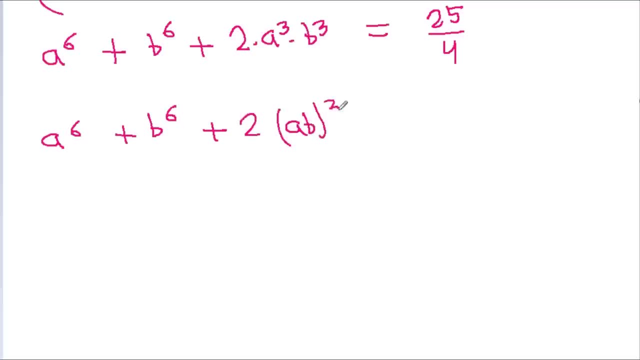 and a cube. b cube is a, b whole cube. that is equal to 25 by 4 and it is a power 6 plus b, power 6 plus two times and a- b is minus 1 by 2. cube is equal to 25 by 4 and it is: 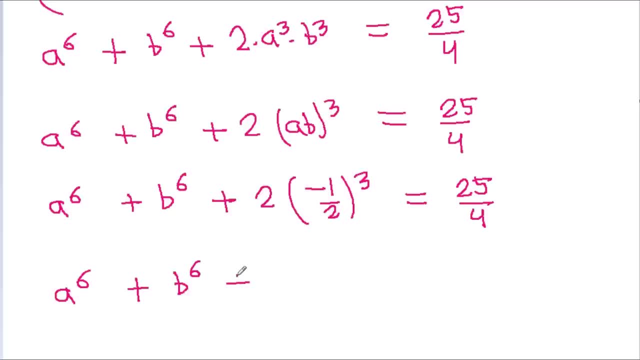 a power 6 minus b power 6 minus 2 times minus 1 by 2. whole cube that is equal to 25 by 4. cube is minus 1 by 8. that is equal to 25 by 4 and it is a power 6 plus b power 6 and 2 times minus. 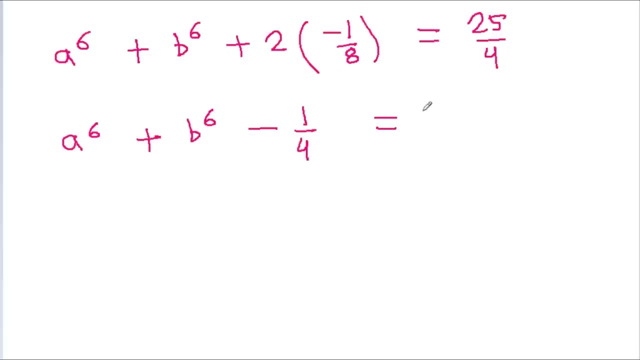 1 by 8 is minus 1 by 4, that is equal to 25 by 4, and a power 6 plus b power 6 is equal to 25 by 4. plus 1 by 4 will be 26 by 4 and we get a power 6 plus b power. 6 is equal to 26 by 4 is 13 by 2.. 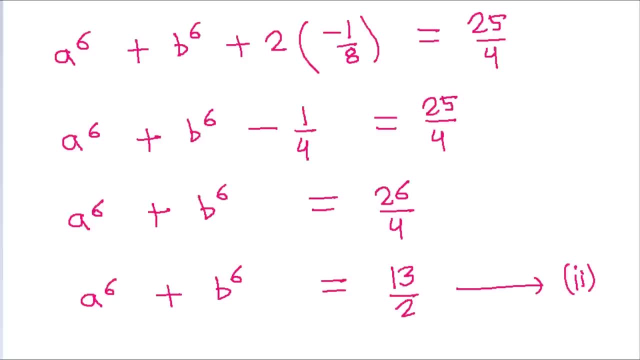 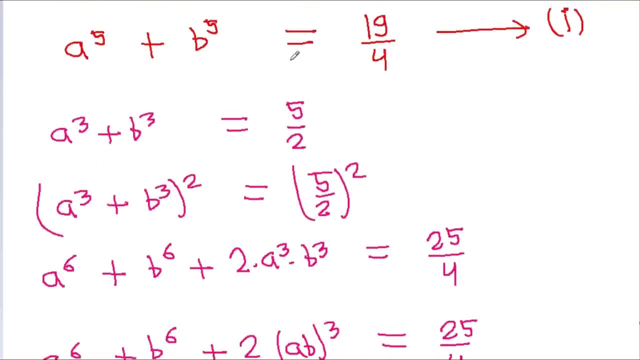 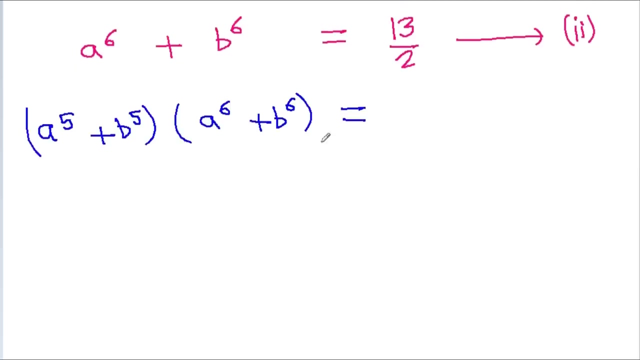 suppose this is equation 2 and if we multiply a power 5 plus b power 5 and a power 6 plus b power 6, then a power 5 plus b power 5 is equal to 19 by 4. a power 5 plus b power 5 is 19 by 4, and a power 6 plus b power 6 is 13 by 2 and a power 5 times a. 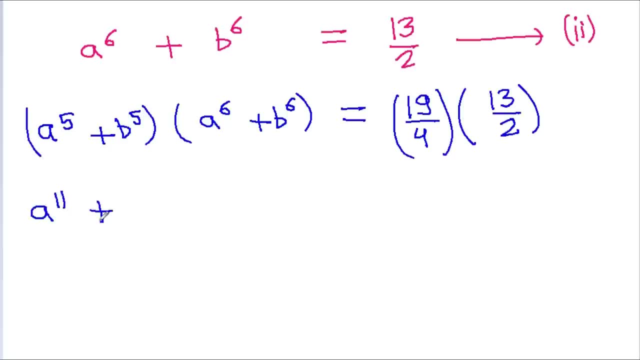 power 6 will be a power 11 plus a power 5 times b power 6 is a power 5. b power 6 minus b power 5 times a power 6 is b power 5. a power 6 plus b power 5. 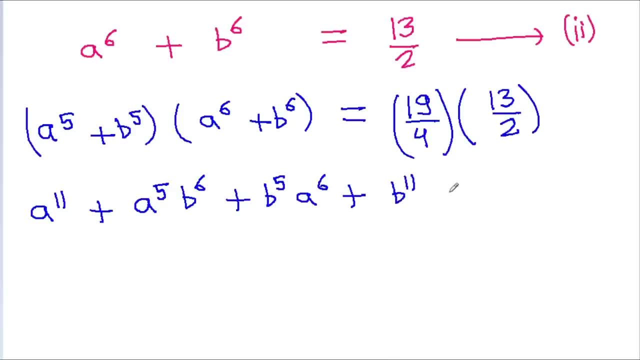 times b power 6 is b power 11. that is equal to 19 times 13, is 247. by 4 into 2 is 8 and it is a power 11 plus b power 11 plus, and from these two terms we can take a power 5 and. 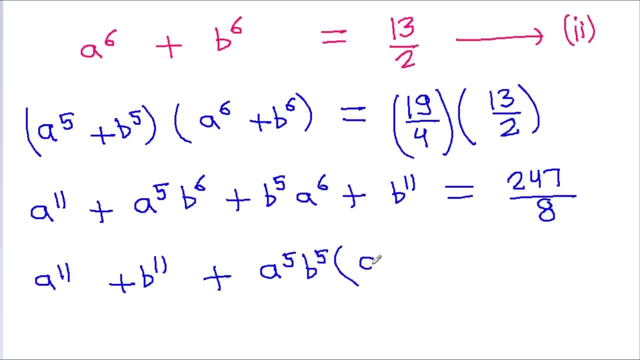 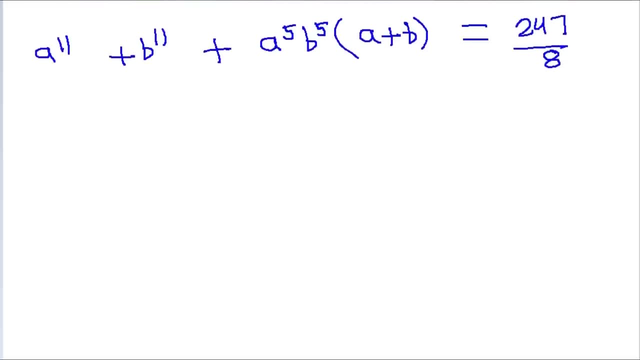 b, power 5 common and we will get a plus b. that is equal to 247 by 8 and it is a. power 11 plus b. power 11 plus a. power 5 times b. power 5 is ab. 1. power 5 times a plus b is equal to 247 by 8 and it is a. 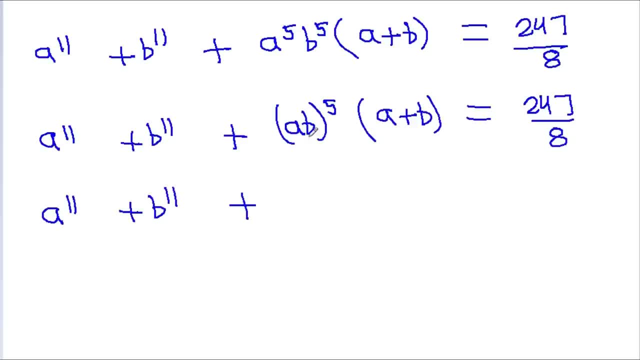 power 11 plus b. power 11 plus ab is minus 1 by 2 power 5, and a plus b is 1. that is equal to 247 by 8 and we get a power 11 plus b power 5.. b power 11 and minus 1 by 2. 1 power 5 is minus 1 by 32, is equal to 247 by 8 and it is a power 11. 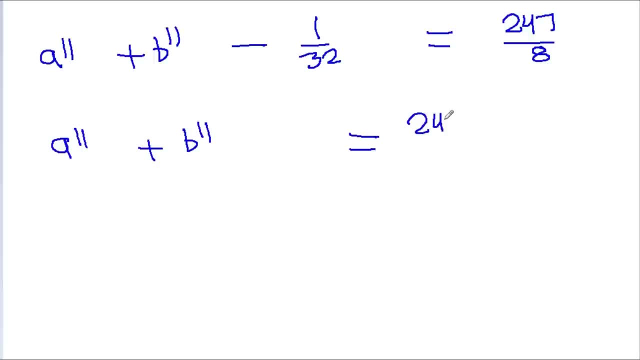 minus b power 11 is equal to 247 by 8, minus 1 by 32 and a power 11 plus b power 11 is equal to 32, will be ncm, and 247 times 4 is 7 into 4 is 28, and 4 times 4 is 16 plus 2 is 18, and 2 times 4 is 8 plus 1 is 9. 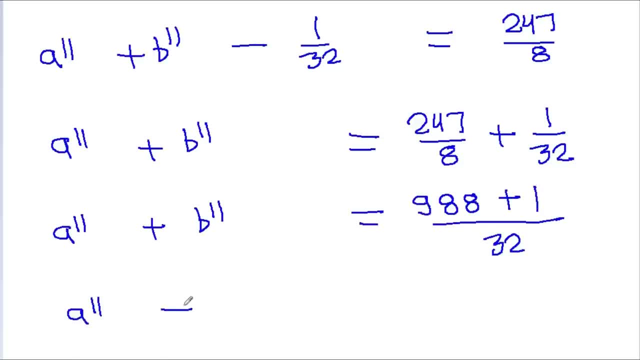 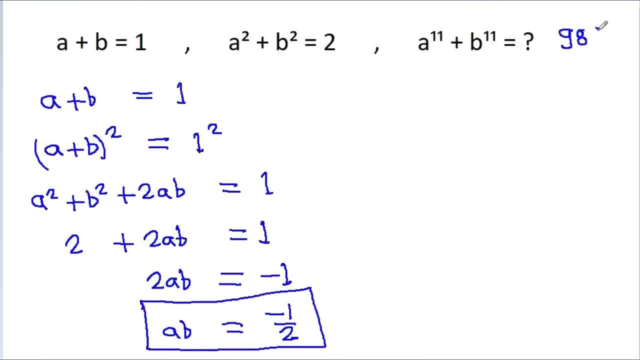 plus 1 and we get a power 11 plus b. power 11 is equal to 989 by 32.. So this is equal to 9 989 by 32.